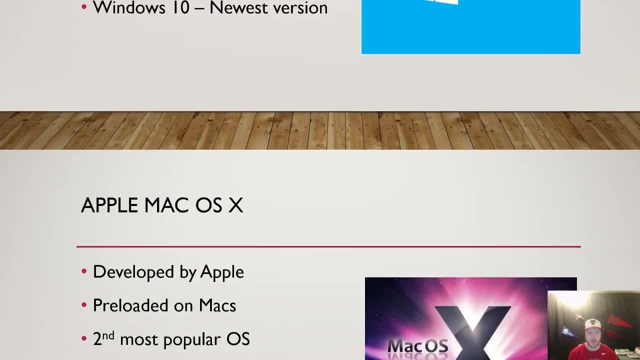 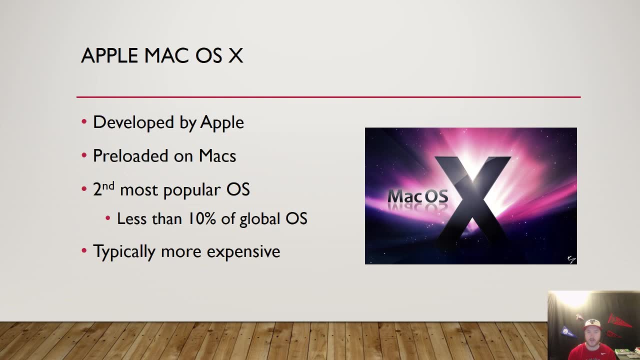 2000.. All right, so the next one I want to talk about comes from Apple, and that's your Mac OS X operating system. Now, this one's developed by Apple and it's pre-loaded onto Macs or MacBooks, and that's. 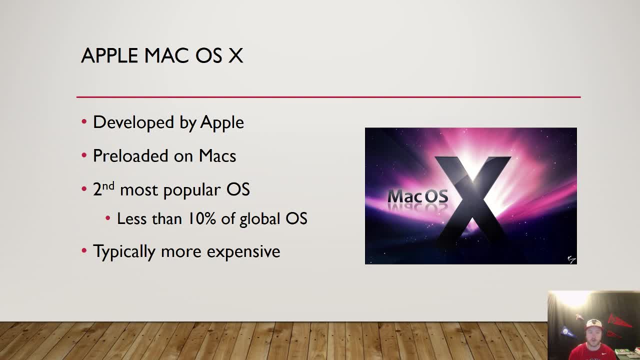 their laptop version. This is the second most popular operating system in the world. Now, if Windows is taking up 80% of the market and Mac is taking up 10%, well, that's obviously a big difference between the first and second largest desktop operating system. 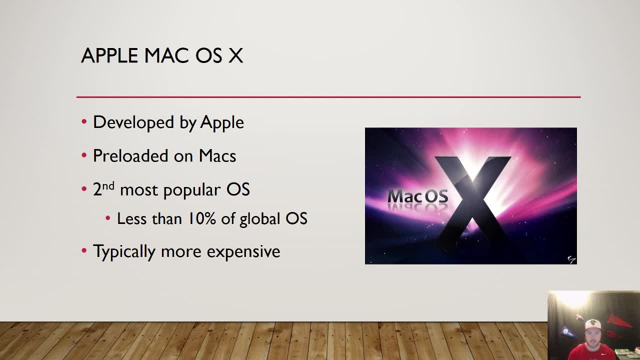 The reason for this is Macs are typically more expensive than your PCs or your Windows 10 computers. Now, if you've ever used a Mac or you've ever used a Windows computer, you will notice that there are some big differences between the two operating systems. I know that every time. 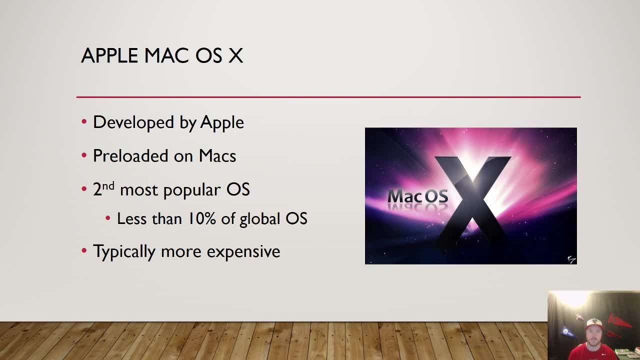 I get on a Mac, I have to really pay attention to what I'm doing, just because I'm not as used to it. So you guys have probably seen some of my other tutorials on Windows 10.. You guys know I'm very familiar with that. 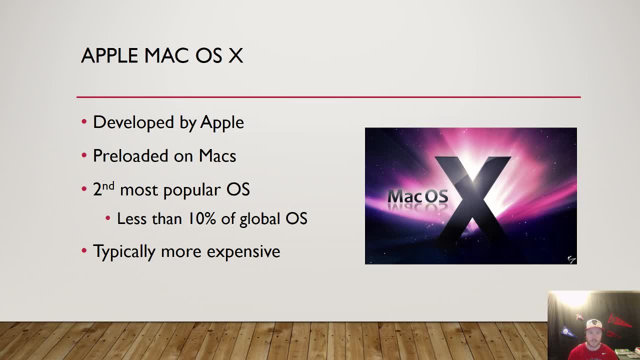 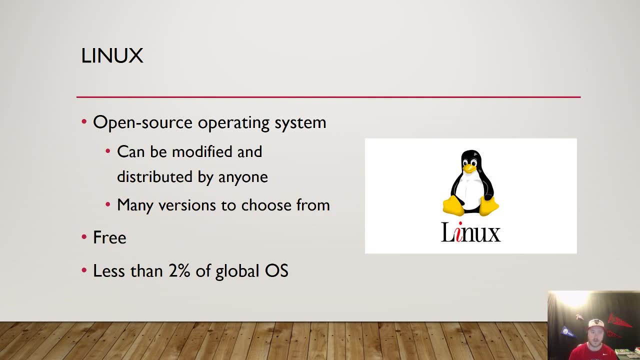 But if I get on my Mac, I'm still learning how to use it, So that's one thing that you do have to know if you ever switch operating systems. Now, the third one that I wanted to talk to you guys about is called Linux, And Linux is an open source operating system, meaning it can be modified, and 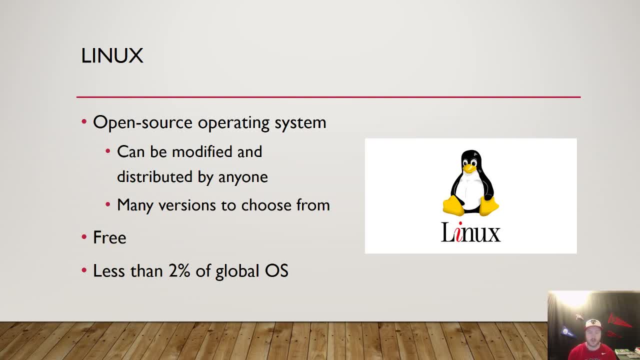 distributed by anyone. The ability to be open source and the fact that it's open source means that many versions are available on Linux. So many versions and many servers run Linux because it's relatively easy to use as far as software goes. So another advantage of Linux is that it's free. But the thing is 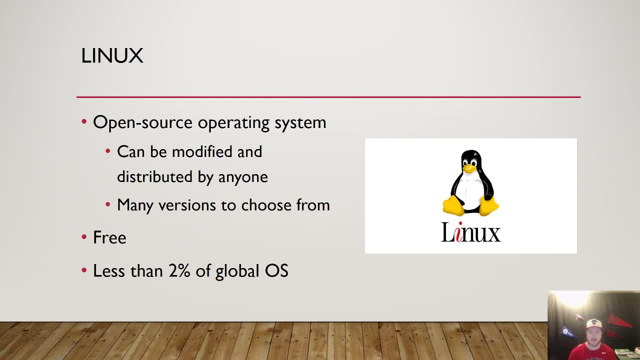 this is the third most popular operating system and less than 2% of global operating systems are currently using Linux, So if you're looking for a free option with many versions to choose from, you may want to go with a Linux operating system. So those are your top three most popular desktop. 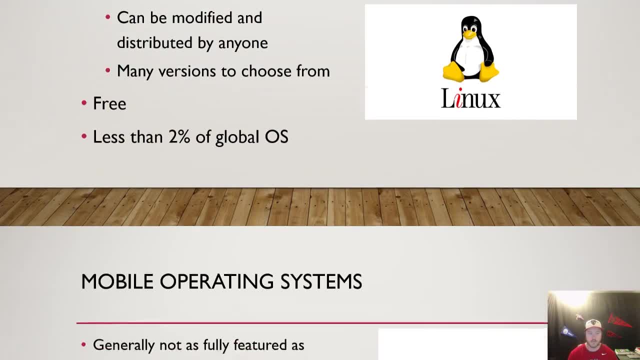 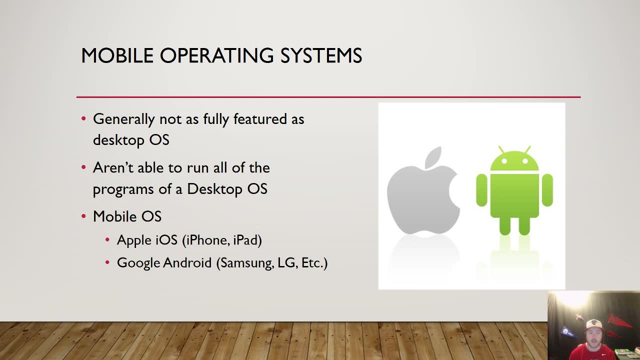 operating systems. Next, we're going to look at mobile devices. Okay, so if you use a mobile device, you know that your mobile device is generally not as full featured as your desktop. For instance, if you have Microsoft Excel downloaded on your phone, you're going to notice that it's a lot easier to use on your PC or on your Mac.